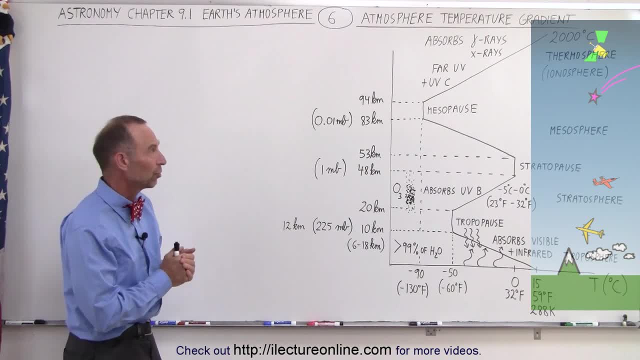 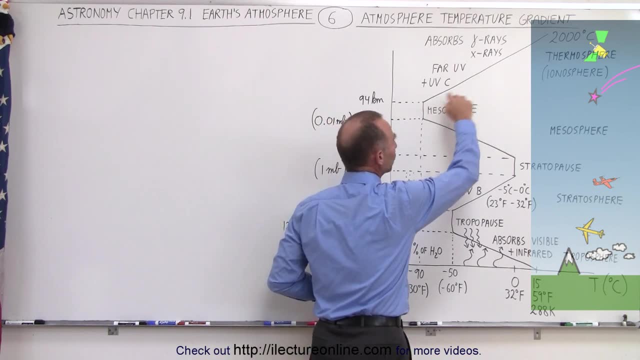 molecules are being ionized by the high energy radiation that reaches the Earth's atmosphere. Notice we see these lines going back and forth and those lines are what we call the temperature gradients. It is warmer to the right and colder to the left. so you can see here that from the 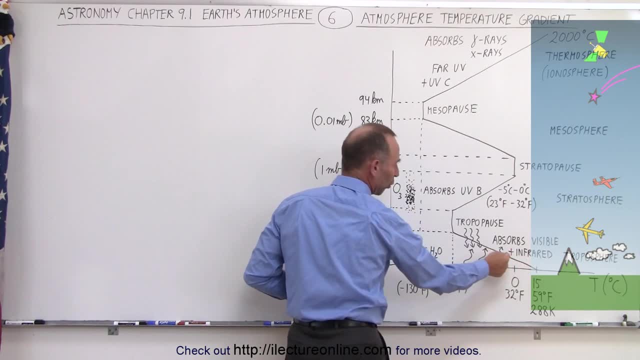 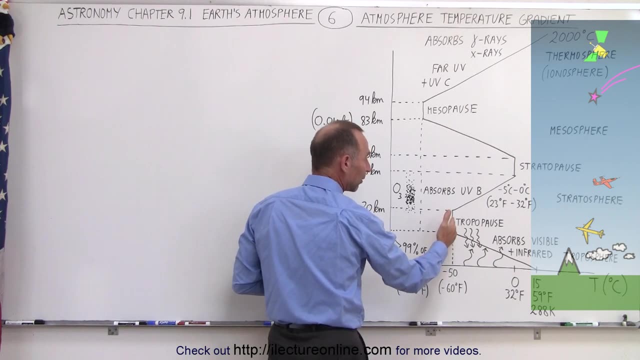 Earth's surface. as we go up into the atmosphere, the temperature gets colder and colder and colder. But strangely enough, at some point that temperature gets colder and colder and colder, That temperature gradient stops For a while. the temperature stays about the same, and then, as we 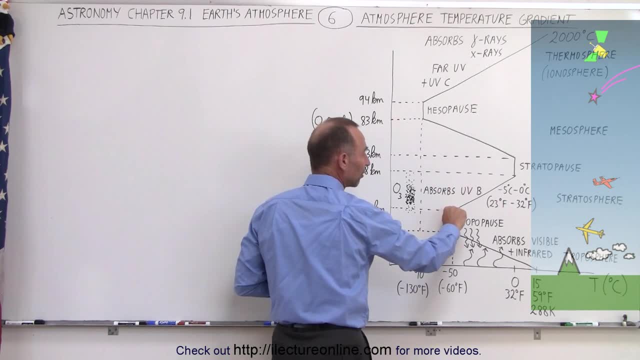 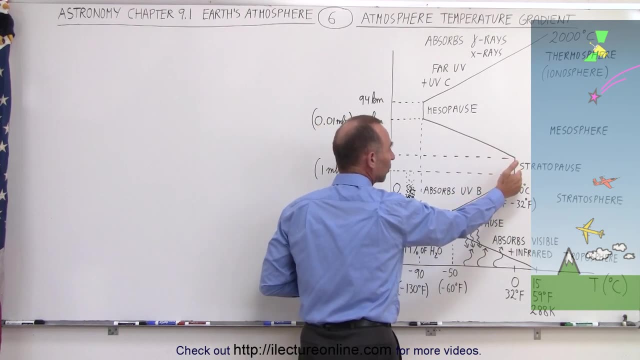 continue to gain elevation or altitude into the atmosphere. the temperature begins to reverse. It starts getting warmer and warmer and warmer again in the stratosphere. Then again that increase stops For a while. there it stays about the same. Then the temperature begins to decrease. again, and this time it gets even colder by the time we reach the top of the mesosphere compared to the top of the troposphere. Then the temperature stays about the same for a while And then it becomes warmer again, because in the very upper portion of the atmosphere. that is where the atmosphere absorbs much of the high energy radiation, such as gamma rays, x-rays, far UV and UV-C that enters our atmosphere. So the absorption of those very high energy rays do heat up what we call the thermosphere And that's part of the reason why they call it the. thermosphere, the heat region or the heat band of the Earth's atmosphere. Notice, we have these three regions where the temperature doesn't seem to be changing much as we gain in elevation, And so we call that the tropopause at the top of the troposphere, the stratopause at the top of the stratosphere. 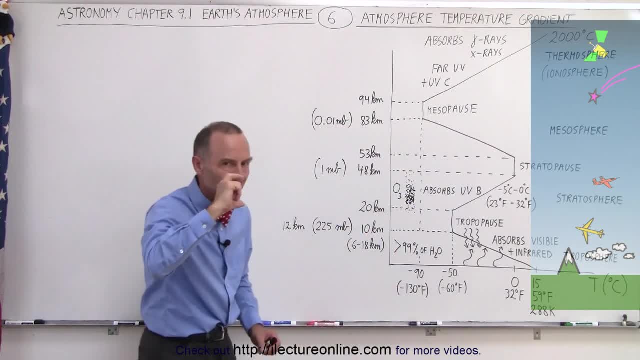 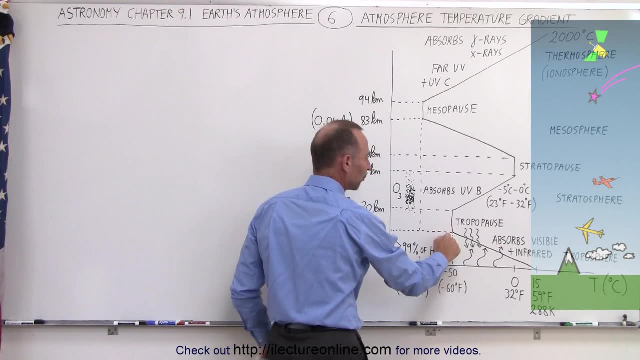 and the mesopause at the top of the mesosphere, Just indicating that there's a region there where there's not a lot of change in the temperature, Notice by the time we reach the top of the troposphere, this is pretty well where all of the Earth's climate takes place: all the clouds. It also contains more than 99 percent of all the water vapor, And so in that region, when we get to the top of it, the temperature drops to about minus 50 degrees centigrade, about minus 60 Fahrenheit. It varies a little bit, depending. upon where on the Earth you are and whether or not it's summer or winter in that region. Notice that the height of the troposphere varies anywhere from about six kilometers, about four miles, at the poles, to as much as 18 kilometers near the equator. So there's. 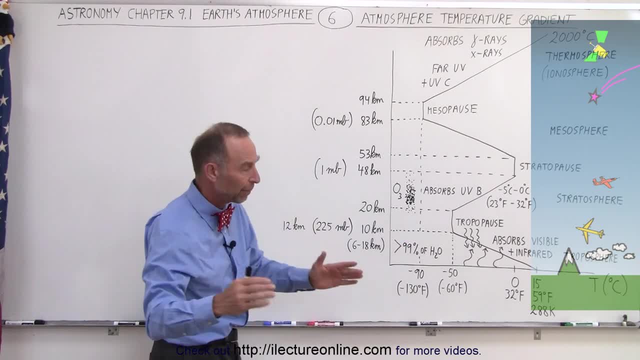 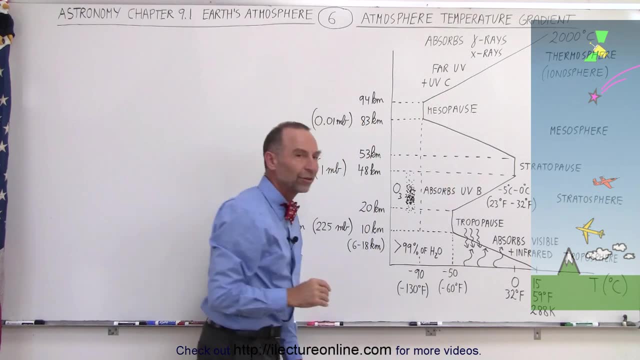 some variation as to where the top of the troposphere is, depending upon where you are in the atmosphere. Now, why do we have these various gradients in the temperature? Well, we already explained that at the very top. the reason why it gets so hot- as much as 2000 degrees. centigrade in the thermosphere is because it absorbs so much of that high energy radiation from space and from the sun And even though it appears like it's really hot, you might burn yourself by going to that region. the air is so rarefied over there that you really don't feel it. 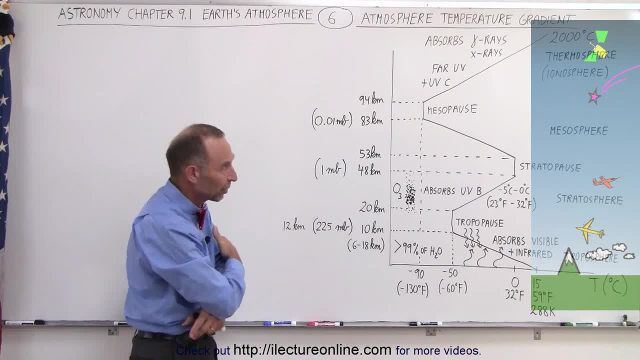 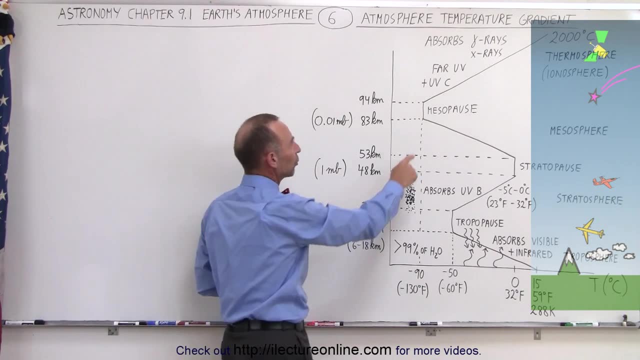 If you had your skin exposed to that temperature, you'd still feel very, very cold because of the radiation into space and you wouldn't get a lot of heat from the very fast moving molecules. Notice it gets very cold by the time you get to the top of the mesosphere here. 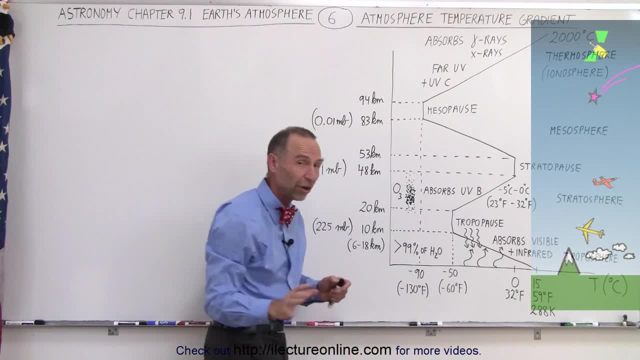 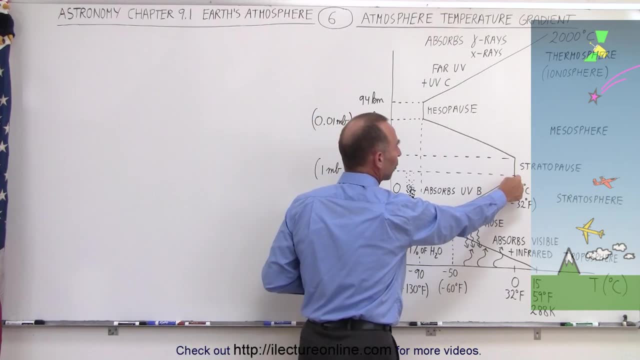 the temperature is about minus 90 degrees centigrade, which is about minus 130 degrees Fahrenheit. very, very cold. But then you can see at the top of the stratosphere it is a lot warmer. the temperature reaches almost zero degrees centigrade. 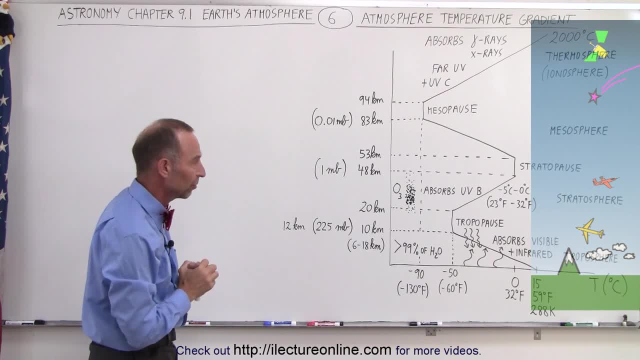 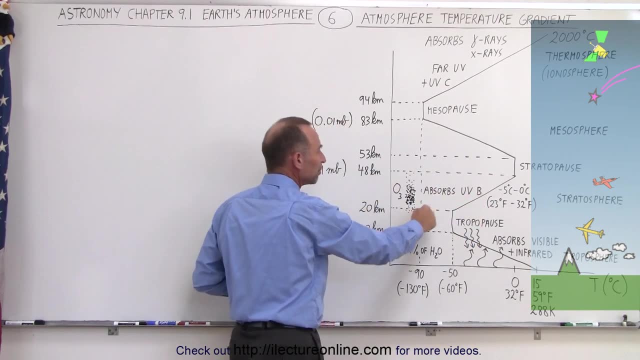 almost 32 degrees Fahrenheit, somewhere in the 20s, presumably Now. the reason why that's happening is in the stratosphere. this is where we find most of the ozone, the O3 molecule, which is most dense, near about the one-third height between here and here into the stratosphere. We find ozone all the. 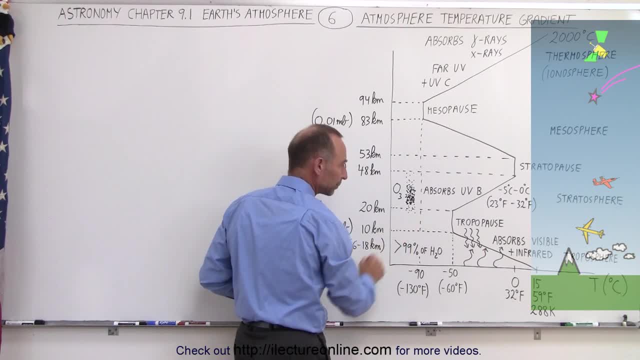 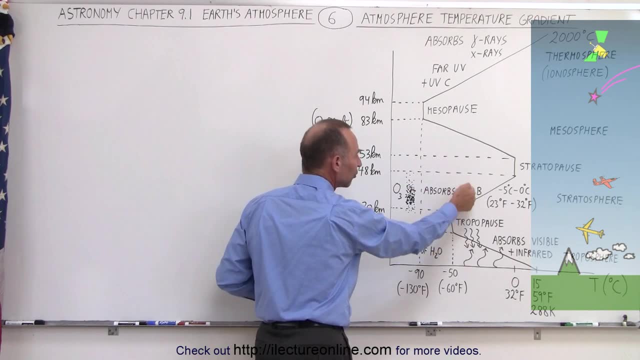 way throughout the stratosphere and a little bit into the troposphere perhaps, and maybe a little bit into the stratopause here, However, most of the UVB is absorbed in this region, right here, and because that contains quite a bit of energy coming from the sun, the temperature gets quite a bit warmer here than 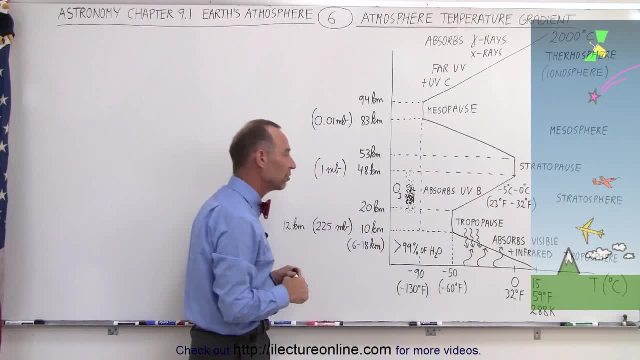 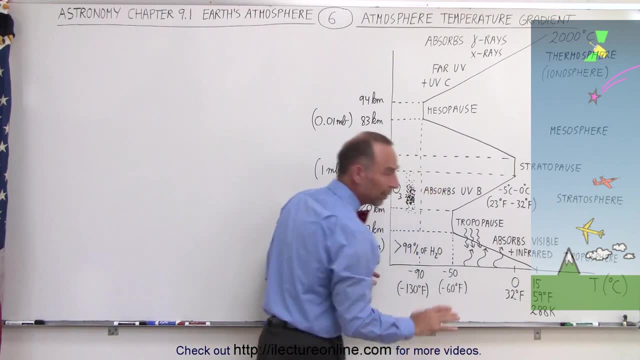 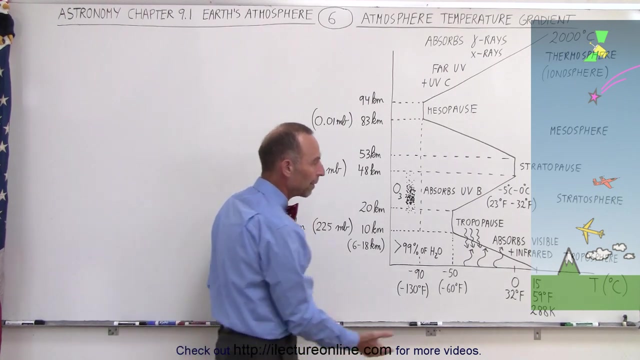 it otherwise would be if it wasn't absorbing this UVB radiation. And finally, the troposphere is nice and comfortable, reaches an average temperature about 15 degrees centigrade, about 59 degrees Fahrenheit. This is day, night at the poles, at the equator, everything averaged out. 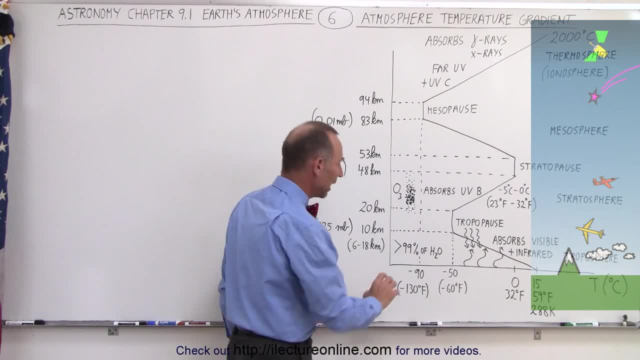 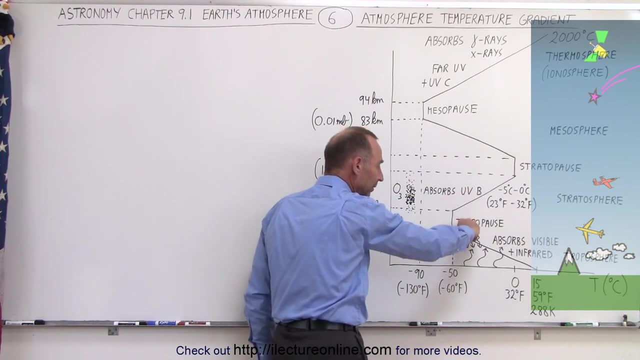 about 280 degrees centigrade. This is a very nice, comfortable temperature, and this is because a lot of the heat that we receive from the sun is absorbed in the troposphere either on the way down or on the way back up from the earth's surface. Notice that the radiation that comes from the earth's surface has 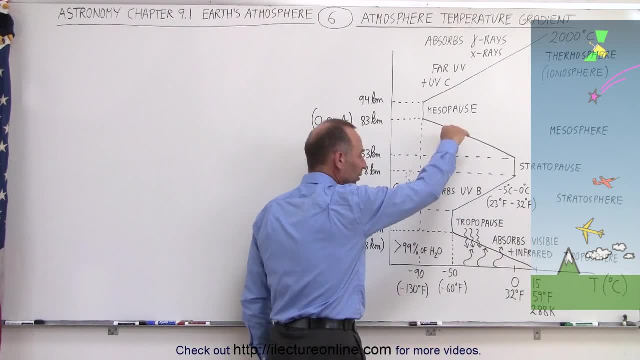 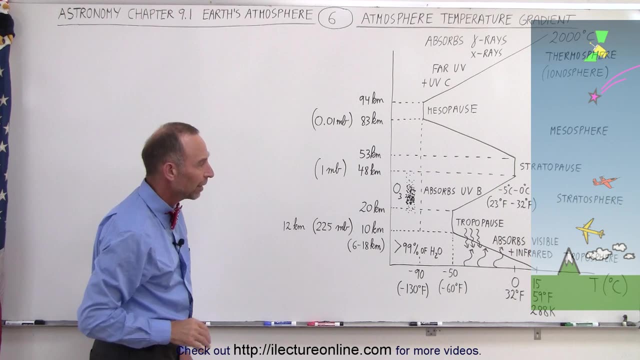 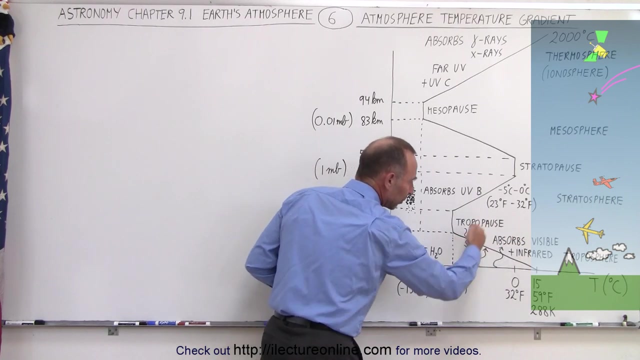 much longer wavelengths, so that's mostly in the infrared. The energy coming down from the sun is mostly in the visible light region, a little bit of, maybe, UVA and a little bit of near infrared. but the net effect is that the radiation that we get from the sun is mostly in the visible range. 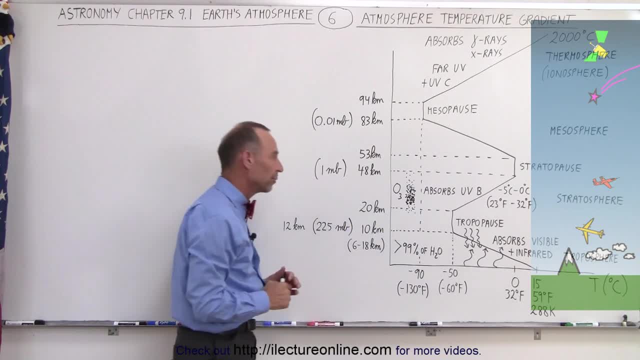 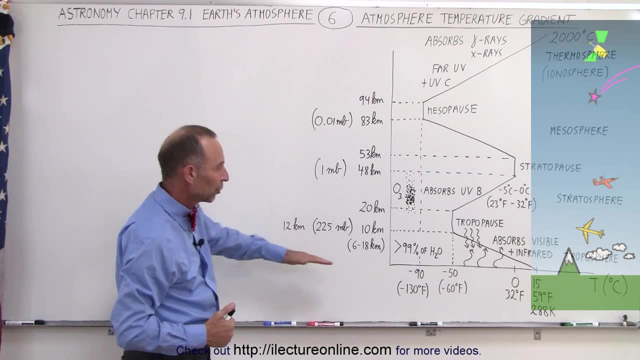 and the radiation coming back from the earth's surface is mostly in the infrared range. So we can see here that there's a lot of relationship or a lot of dependency between the temperature, the various layers and the kind of energy that's being absorbed within the different layers of the 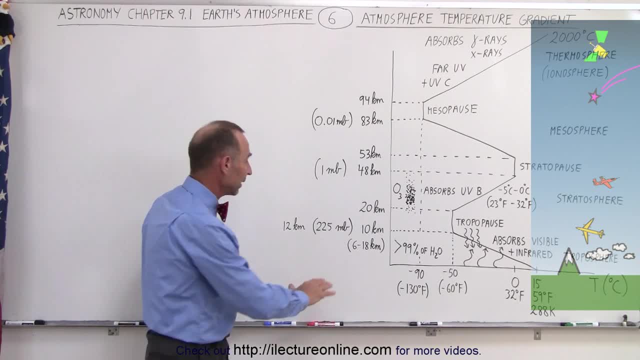 earth's atmosphere- Something interesting to note as well- that the pressure drops quite a bit from the surface at the surface and center of the earth. But again, when you look at the antiquity then it doesn't stop there. But what we're seeing here is that any potential CDC decision based the pressure of the atmosphere is around 1,000 millibar- about 1,013 millibar on average. It drops quite quickly to about 225 millibar by the time we reach a height of about 10, 12 kilometers.